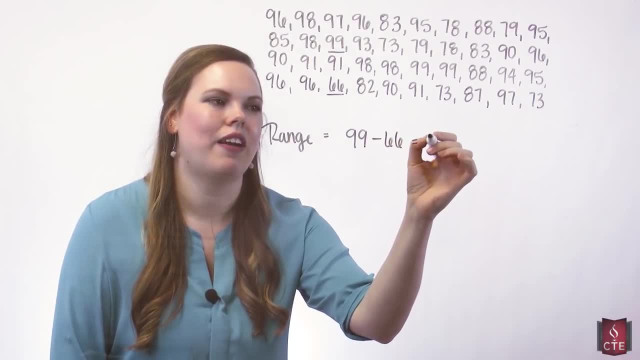 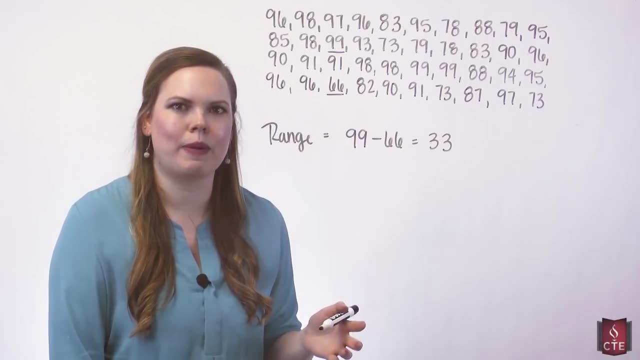 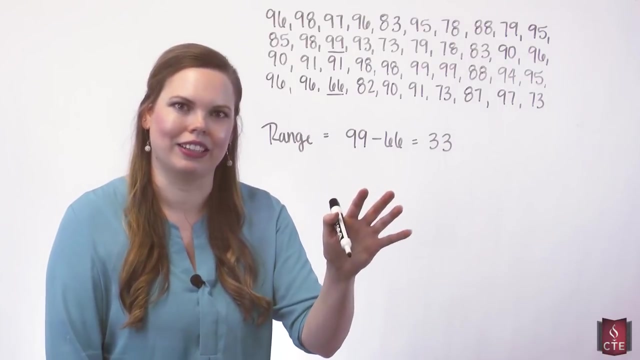 66. We have a range of 33.. So as we think about how many classes that we want, we want to keep in mind that we don't want to spread them out too much and have, you know, 20 classes for a range of 33.. That would be kind of silly. There wouldn't be much data in each class. 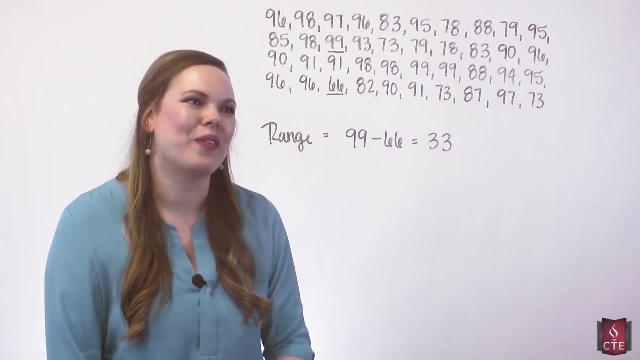 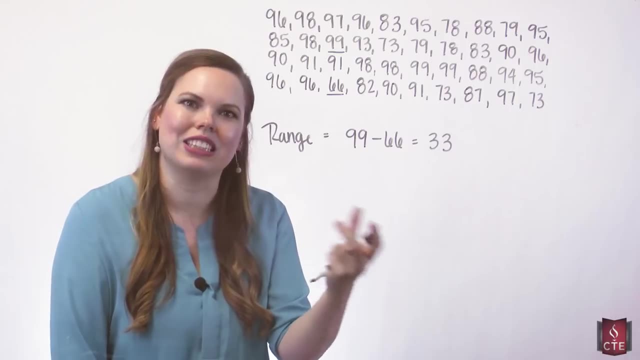 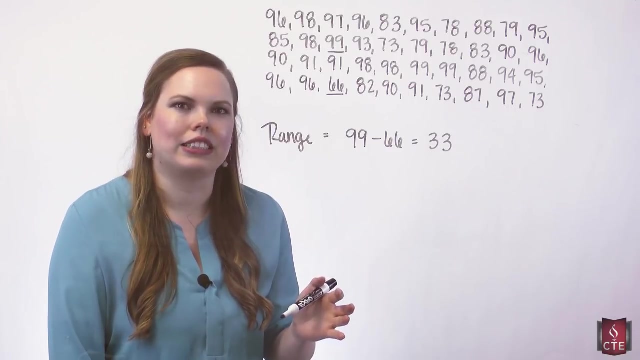 maybe just one or two pieces of data. But we also don't want to get too small, We don't want three classes and then they get all collected into those three classes and we don't see the significant shape of the data either. So but most of the time we want a number of classes, between 5 and 15, as kind of a rule. 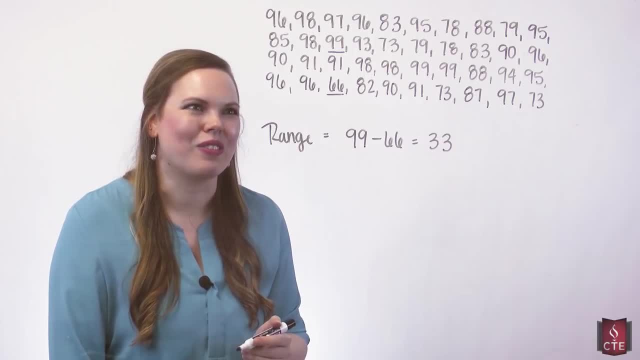 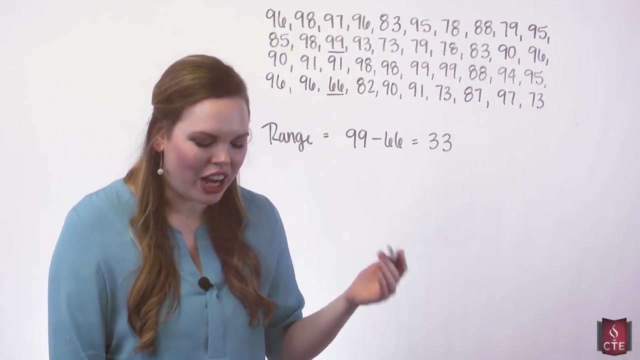 We can bend it, but that's kind of the rule that we deal with when we construct a frequency distribution And for the data that you guys are going to be analyzing in this class, you're probably going to stick around 5,, 6,, 7, maybe up to 10, but probably not. I tried a few. 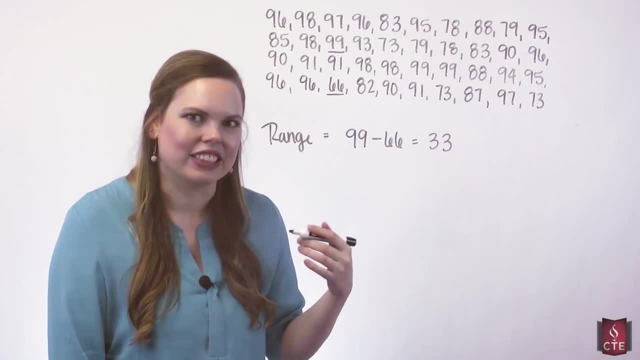 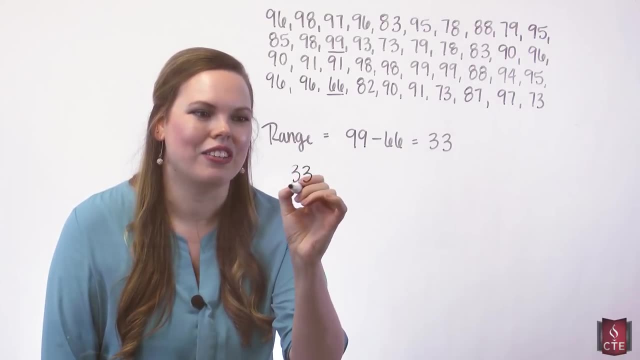 things. I tried 6 and 7, and I landed on 7 pretty quickly because when I took 33 and divided it by 7, this is how you find the class width, which is the next thing you want to do. So this: 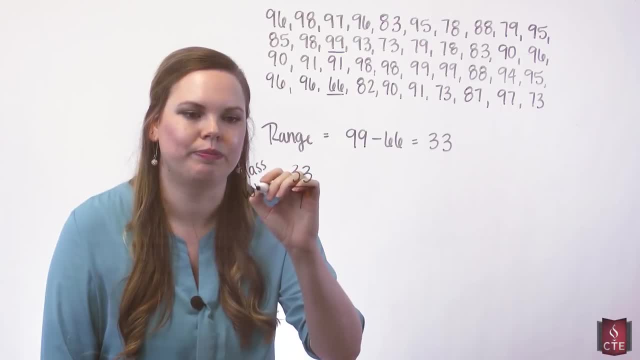 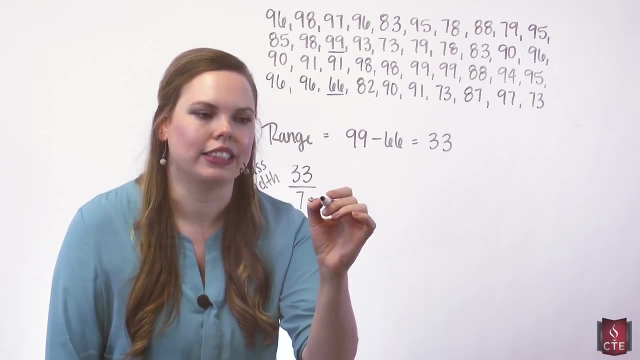 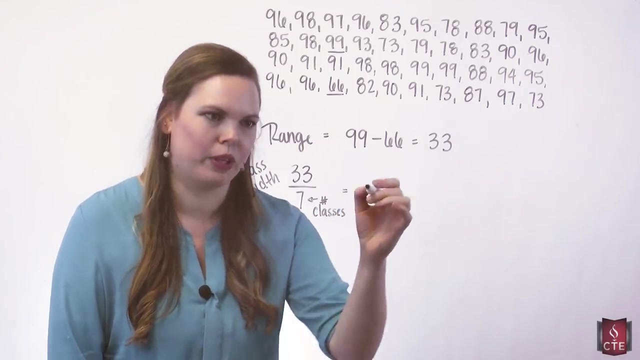 is to find the class width. You take the range and you divide it by the number of classes that you want. When I did 7,, I got 4.71.. And a class width. we put a ceiling function on this And the ceiling means to. 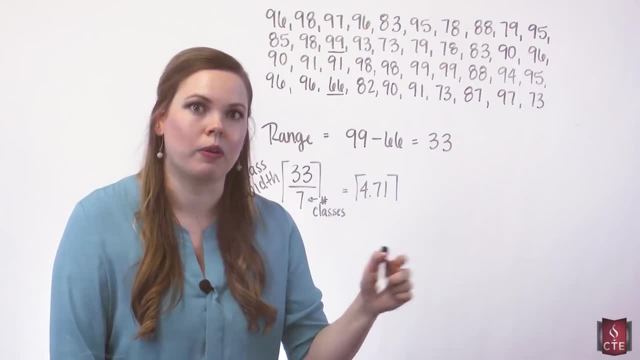 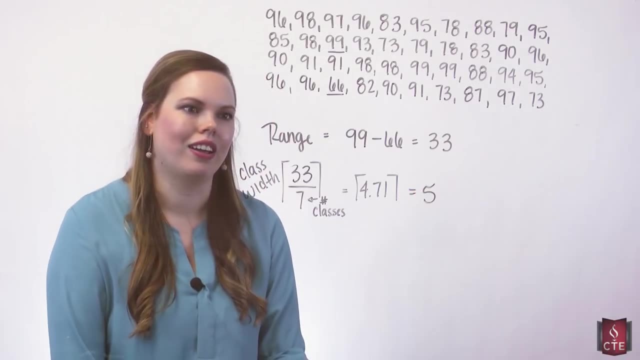 round up the value to the nearest whole number. Always round it up. So even if this was 4.01, we would still round it up to 5, okay, And I like a class width of 5.. It's odd, We like. 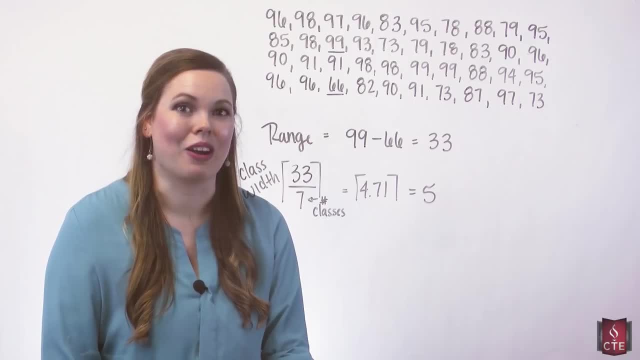 an odd class width, because then our midpoint is a whole number. It's a reasonable value. I like having 5 data values and we just like the number 5.. So I saw that quickly and I was like 7 classes it is So 6,, I think, gave us a 4. And so that was a little bit small for a class width and it was an even number, so I went to 7. And that was what I decided on. 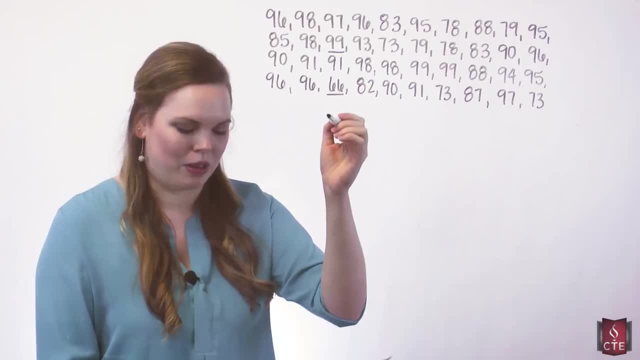 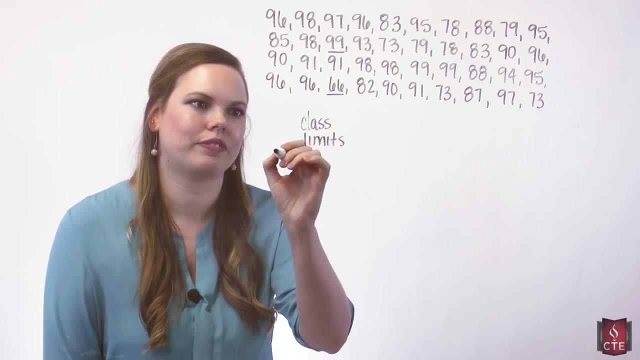 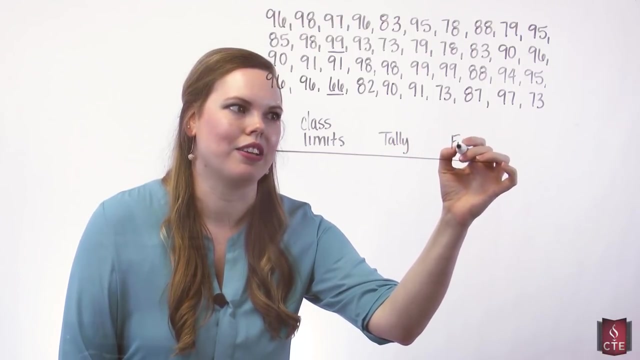 So keep in mind, our class width is 5 and we want to start our class limits for our frequency distribution. So this is our class limit. our frequency distribution also keeps up with a tally. I'll show you why we do that in just a second. and then our frequency. 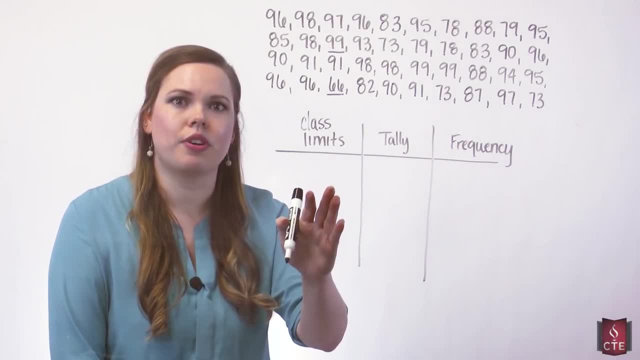 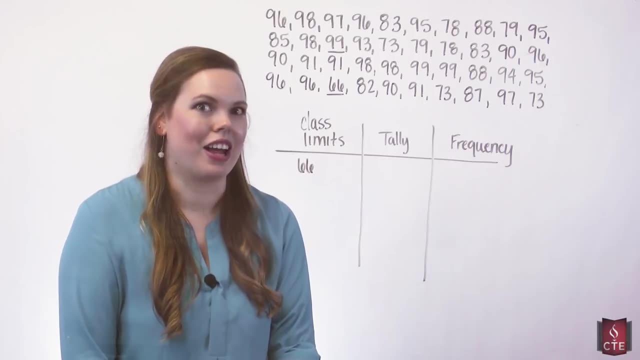 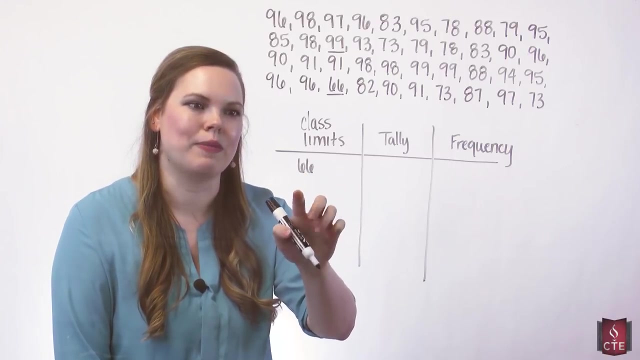 okay, our class limits always start with our smallest data values, so here it would be a 66. our class width is 5, and so the difference between 66 and our net lower class limit it should be 5. so 66 plus 5 is 71. so that's going to be our. 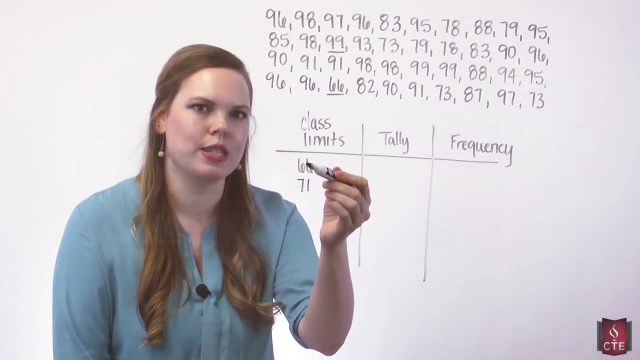 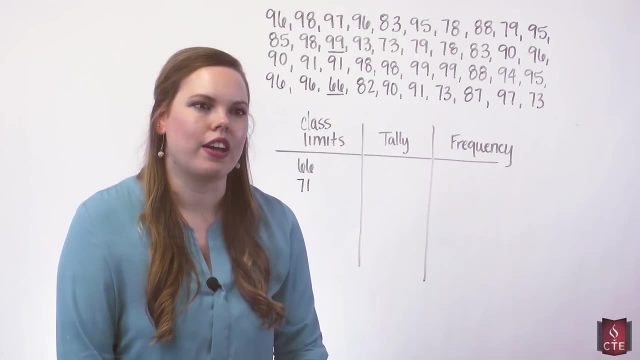 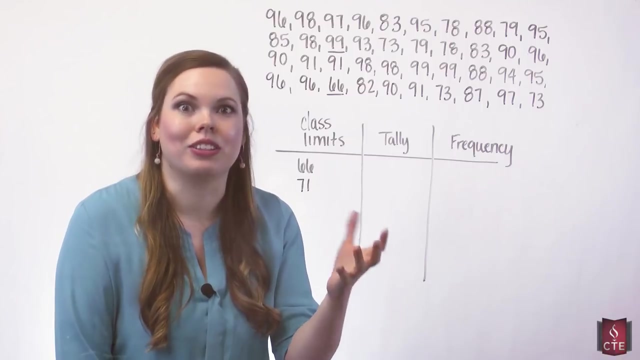 next lower class limit, and the reason why it's this way- vertical and not horizontal- is because we are class. width is the number of data values that are in that class, the number of data. I'm not data values, but the number of numbers that would land right there. so 66, 67, 68, 69 and 70. 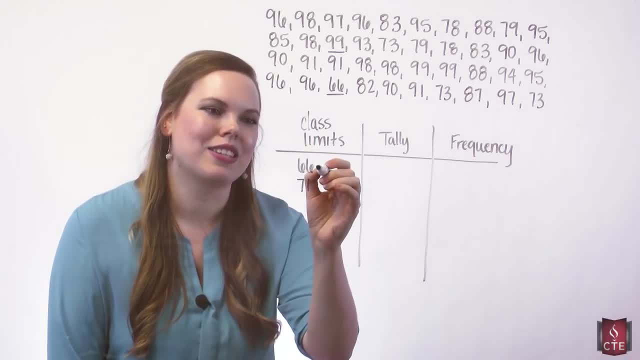 so number of data values. that would land right there. so 66, 67, 68, 69 and 70. So that would land right there. so 66, 67, 68, 69 and 70. So that makes 5, and so that's why this goes up to 70.. 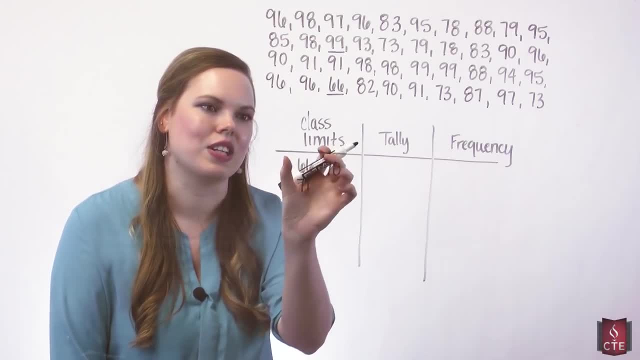 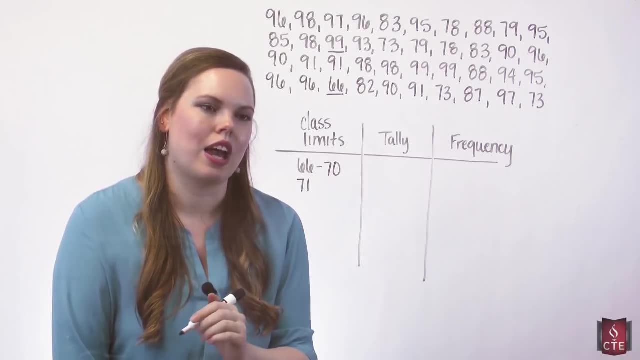 All those values- 66,, 67,, 68,, 69, and 70, is going to land right here, and that's what our class width is representative of. So that's why we're adding 5 vertically as we come up with our class limit. 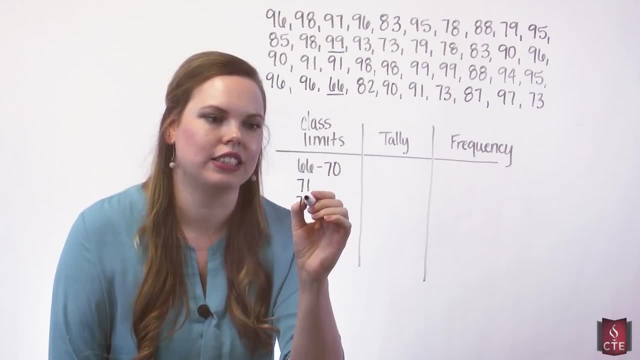 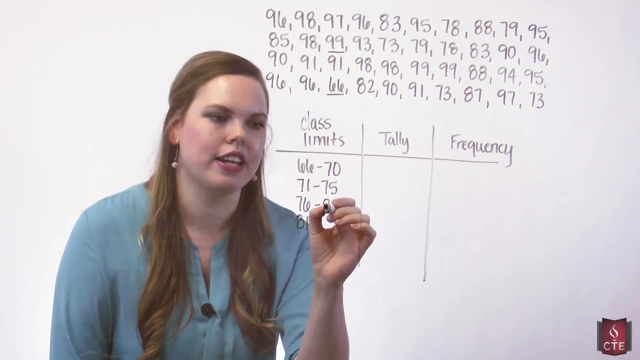 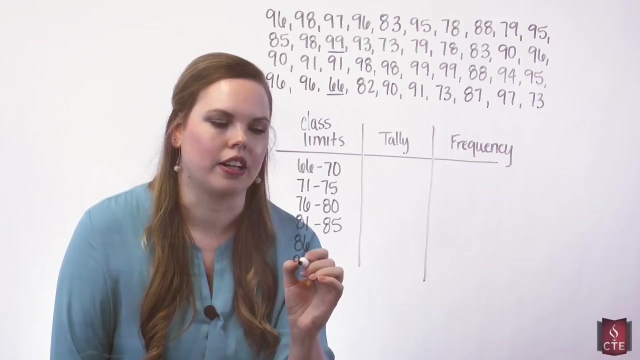 So we'll keep on doing that until we get 7 classes. So 76,, which would make this 75.. 81,, which would make this 80.. 80,, 86,, 91,, 96, and of course that is 7.. 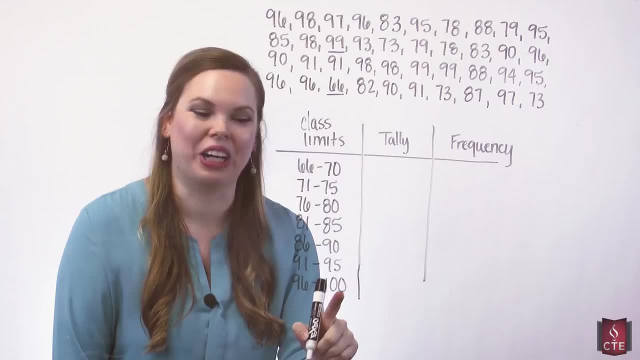 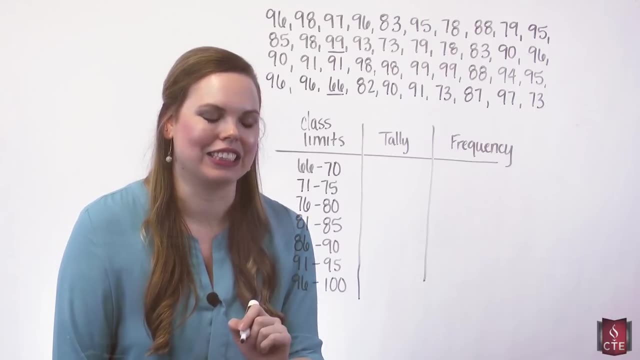 So now we have 7 classes and we of course just add 4 to get to this last, because this would be 101 if we added 5, and so making this last class limit, Upper class limit- 100.. 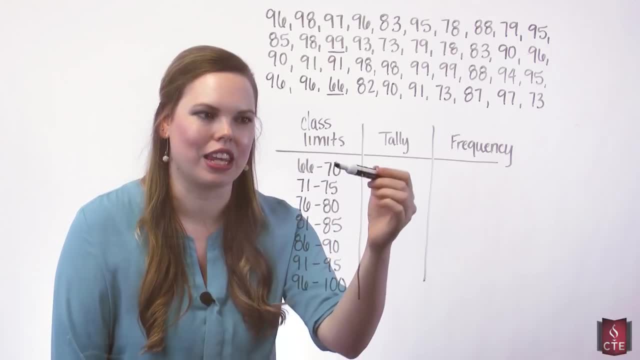 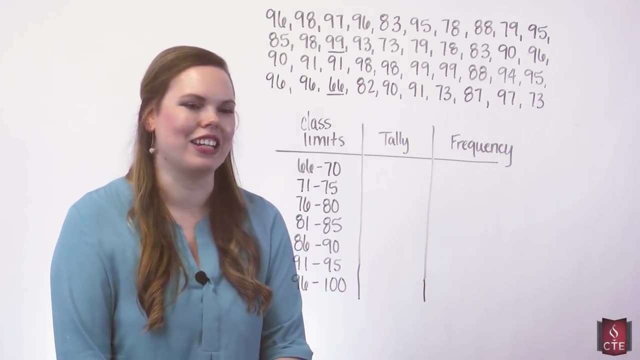 So you can kind of go out down and check. You should be able to add 5 and get to all these, and the difference between all these should be 5, which they end in 5, so that's nice, All right.